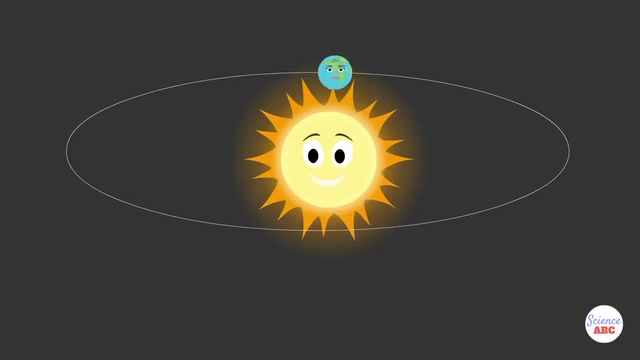 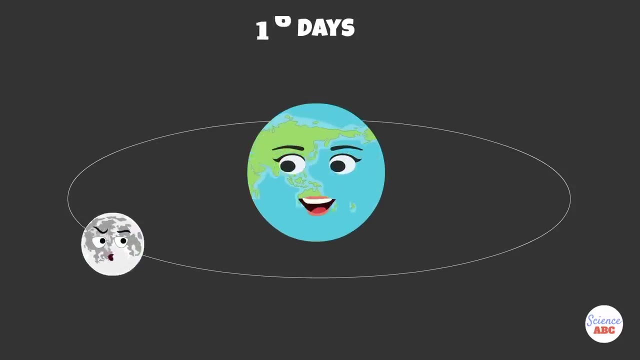 by clicking on the i button at the top right corner of the screen. Just as Earth moves around the sun in an elliptical orbit every year, our natural satellite, the moon, also will revolve around the earth. It takes about 27.322 days for the moon to complete one revolution around our 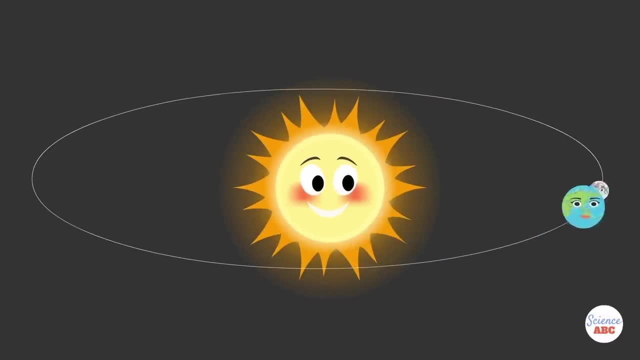 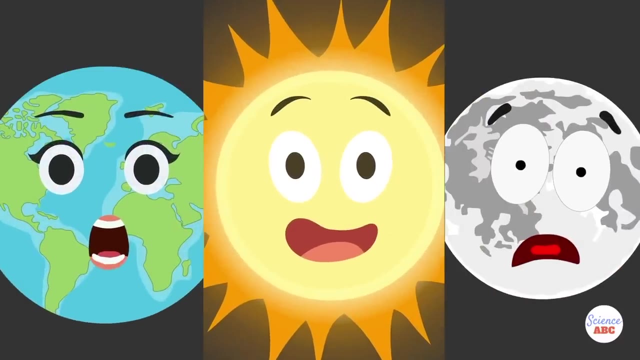 planet. So Earth revolves around the sun and the moon revolves around Earth. Pretty neat, right. Due to all the interrelated motion happening between these three celestial bodies, several physical phenomena occur When the new moon, during its revolution around the earth, 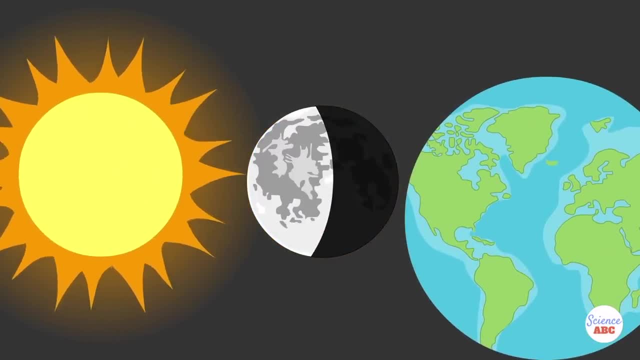 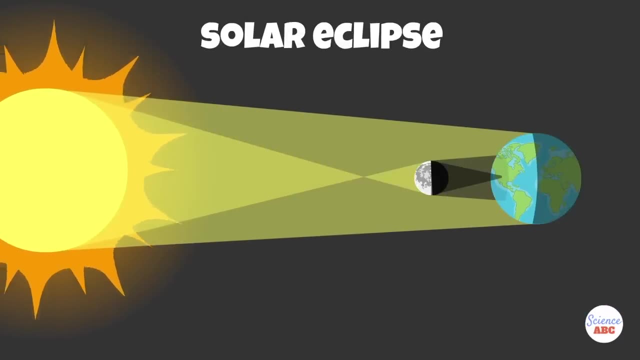 moves between the sun and the earth, it blocks out the sun's rays, which casts a shadow on parts of the planet. This is called an eclipse of the sun or a solar eclipse. In other words, a solar eclipse happens when the moon passes in a direct 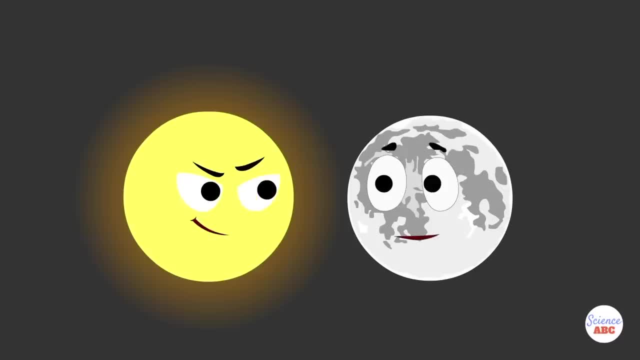 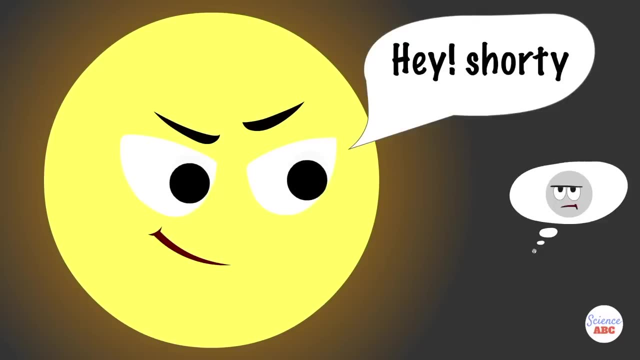 line between the sun and the earth. Now you may be thinking that the moon is infinitesimally small compared to the sun, So why is it ever able to cover part, or sometimes even the entire, sun? Although the moon is indeed about 400 times smaller than the sun, it also happens to be: 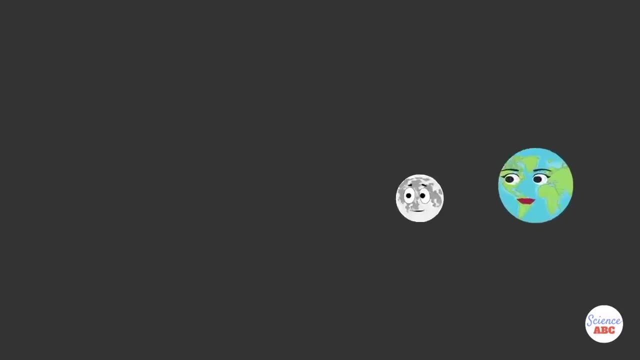 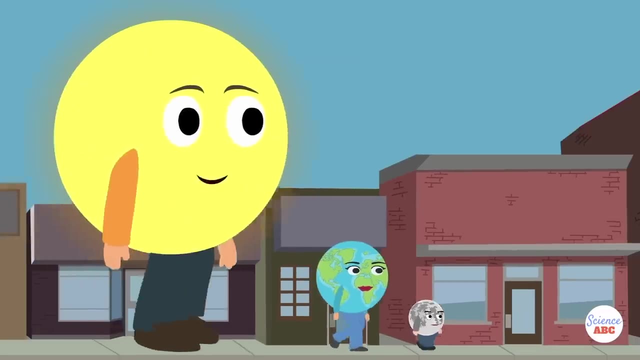 around 400 times closer to us than the sun. This is why both the moon and the sun appear to be the same size in our sky. The moon is very small compared to the the Sun and to the Earth, which is why the Moon's shadow isn't big enough to engulf. 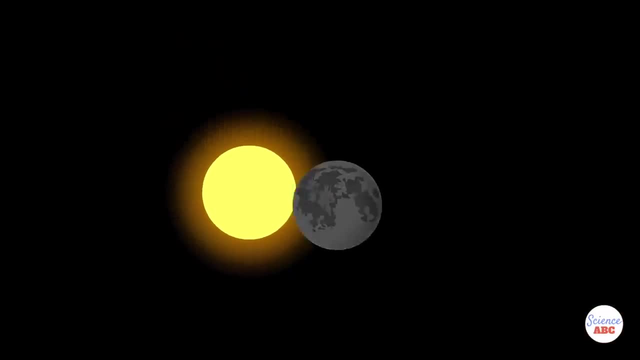 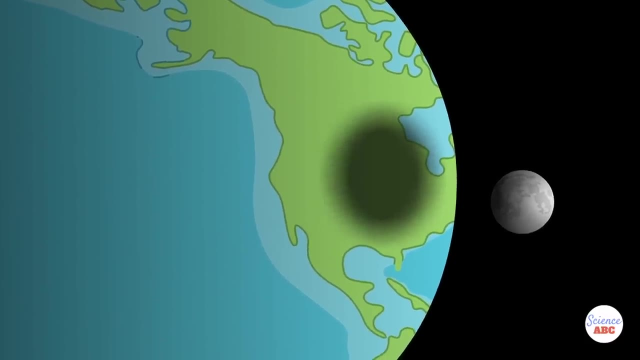 our entire planet. Therefore, the Moon's shadow is always limited to a certain area. This area changes even during an eclipse, as both the celestial bodies are in constant motion with respect to one another. When the Moon eclipses the Sun, it casts two types of shadows on Earth. 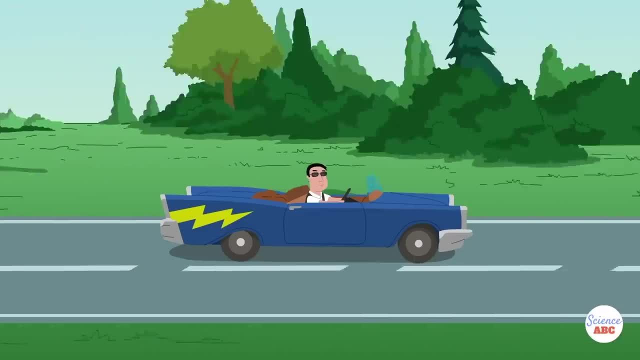 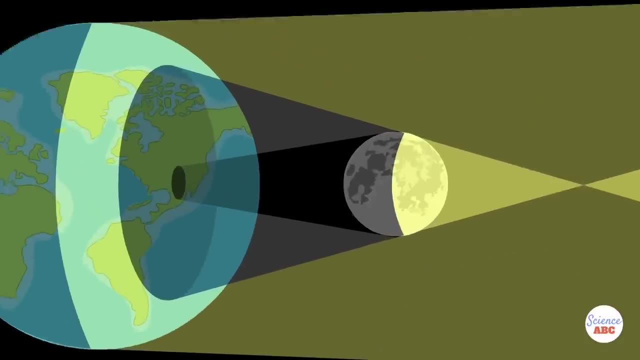 The first is the umbra, which is a small and very dark shadow. If you're in a place on Earth where umbra is cast, the entire central portion of the Sun will be blocked out from your perspective. The second type of shadow is known as the penumbra. 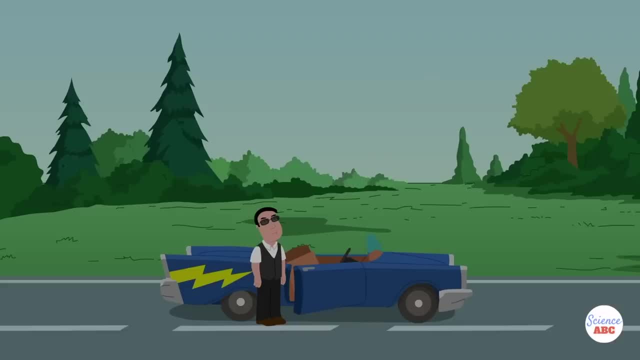 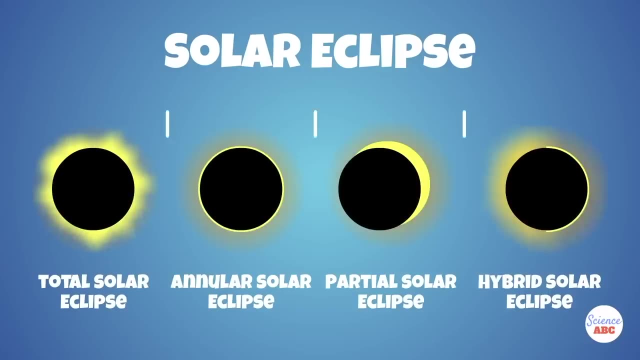 It is a larger and relatively lighter shadow than the umbra. If the penumbra passes over you, then only a small part of the Sun will be blocked out from your point of view, Depending on the type of shadow the Moon casts on Earth. solar eclipses are broadly classified. 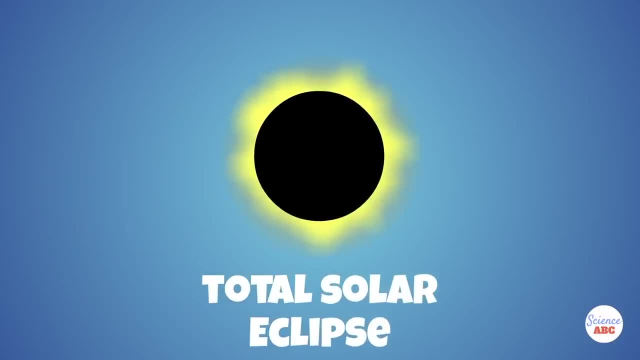 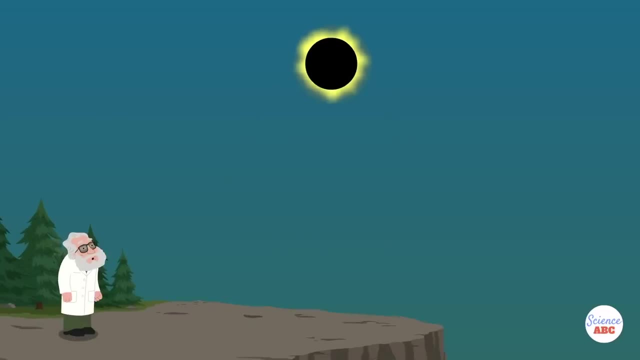 into four types. The first is a total solar eclipse. This is the most spectacular of all eclipses, because during a total solar eclipse, the entire Sun is completely blocked out by the Moon. This can only happen when the Moon is near perigee, the point of the Moon's orbit, when 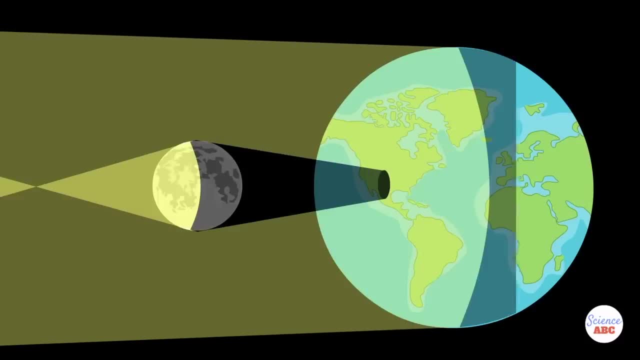 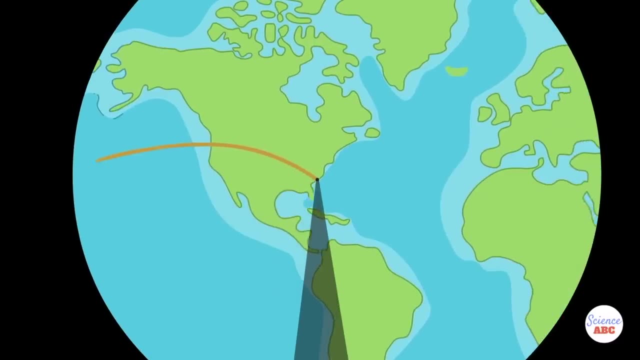 it is closed. You can only see a total solar eclipse if you're standing within the umbral shadow. Since the Earth keeps rotating, the umbral shadow doesn't stay at one point on Earth – it keeps moving too. The imaginary line created by the umbral shadow is known as the path of totality. 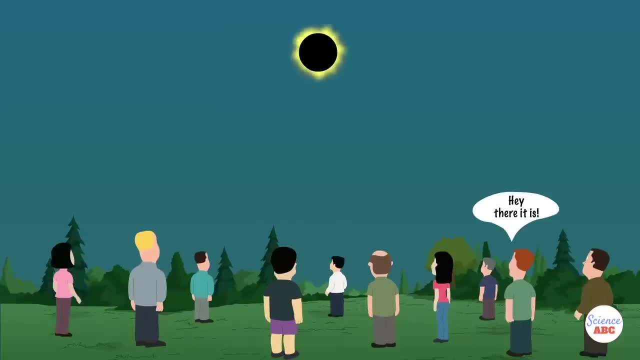 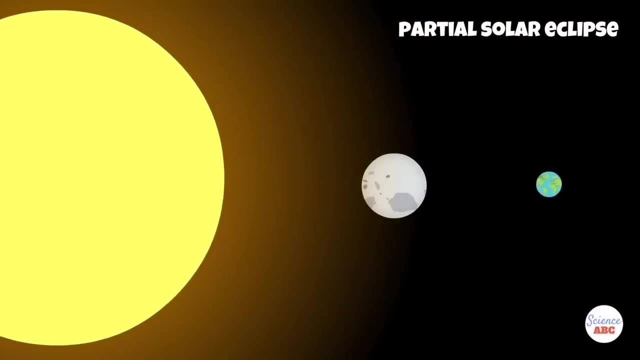 If you're in any of the places through which this imaginary line passes, you can see when the Sun gets completely blocked out by the Moon. Next up is a partial solar eclipse. This type of eclipse is observed when the Moon covers only a part of the Sun and when 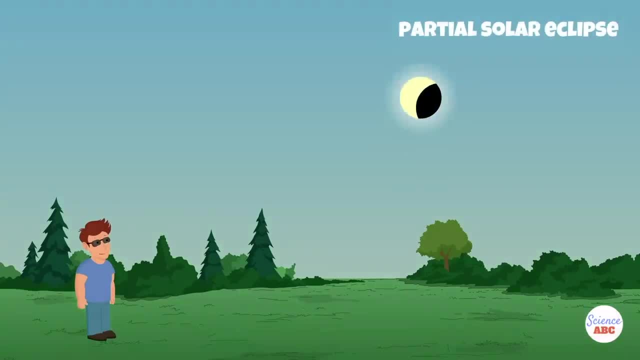 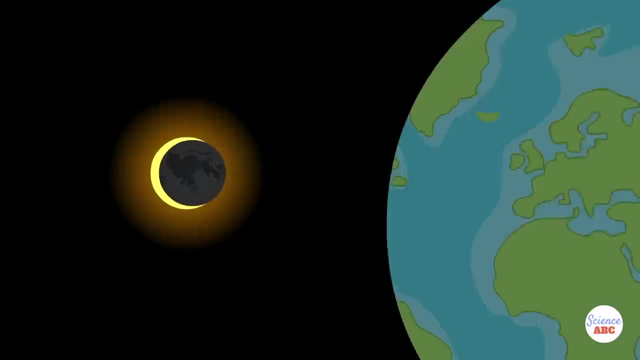 it casts a penumbra on Earth, Since it only covers a part of the Sun. this phenomena is known as a partial solar eclipse. When the Moon passes through the center of the Sun, but its disc isn't big enough to cover the entire disc of the Sun, then an annular solar eclipse occurs. 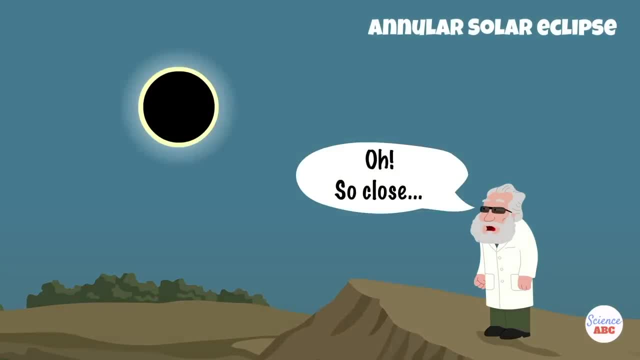 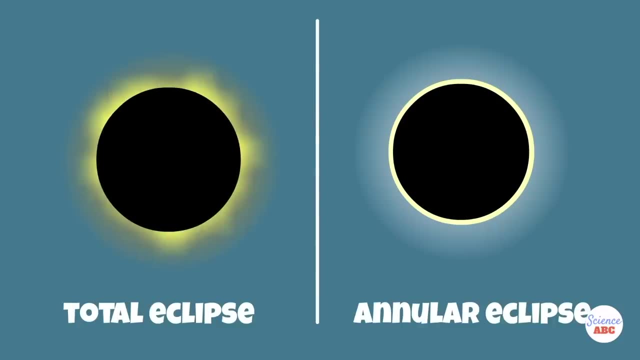 When this happens, the Sun's outer edge remains visible, making it look like a shiny, fiery ring in the sky. Unlike a total eclipse, during an annular eclipse, the Moon doesn't completely block out the Sun. The fourth type of eclipse is called a partial solar eclipse. 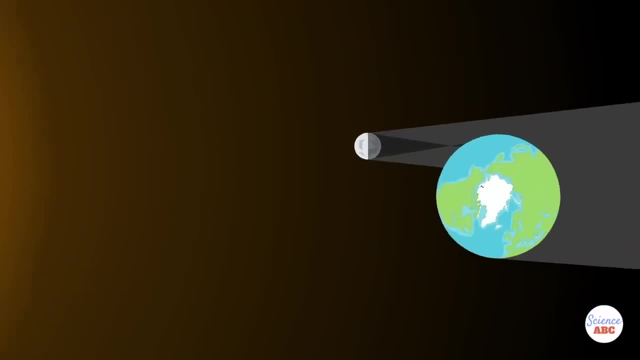 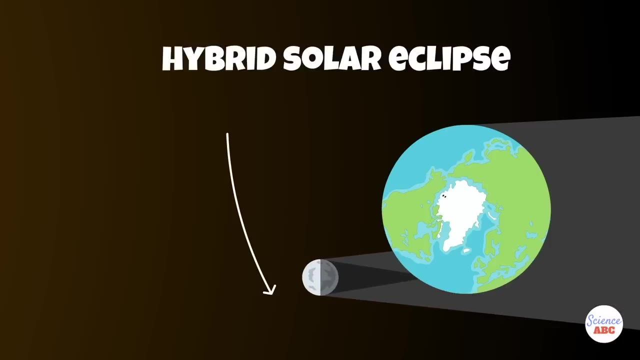 This type of eclipse is the rarest of all. When the Moon's position between the Sun and the Earth is so delicately balanced that Earth's curvature plays a role, we call it a hybrid solar eclipse. During this type of eclipse, some parts of the Earth witness an annular solar eclipse. 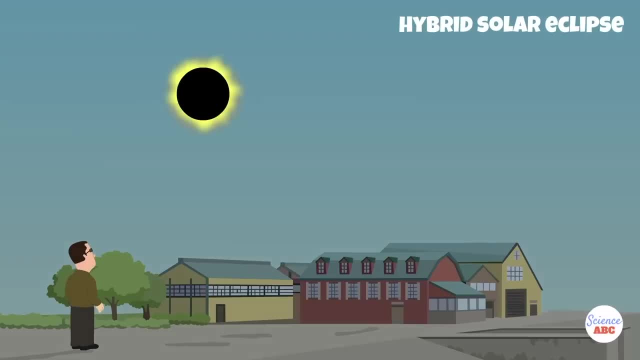 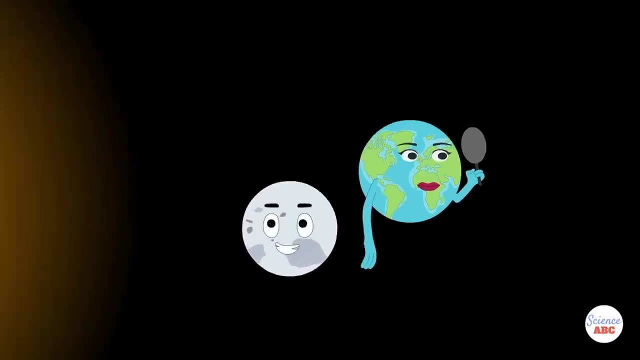 while other parts see a total solar eclipse. For that reason, this type of eclipse is also known as an annular total solar eclipse. Since the Moon continually revolves around the Earth, it's only natural that it sometimes comes between the Sun and the Earth, while at other times it goes behind the Earth. 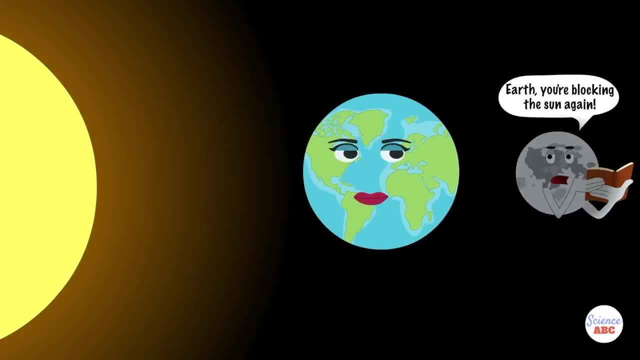 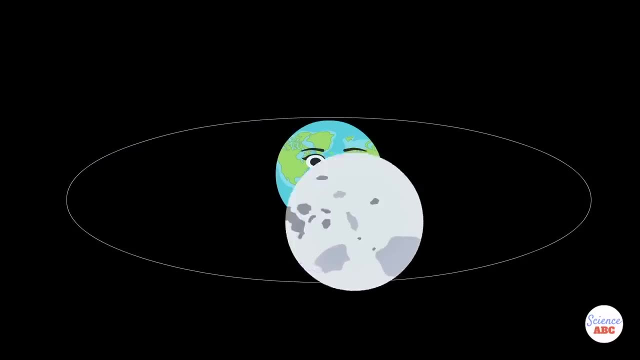 so that the Earth comes between the Moon and the Sun. When the latter happens, we see a lunar eclipse. The Moon completes one revolution around our planet in approximately 27 days and rotates at the exact same rate as it revolves around the Earth. 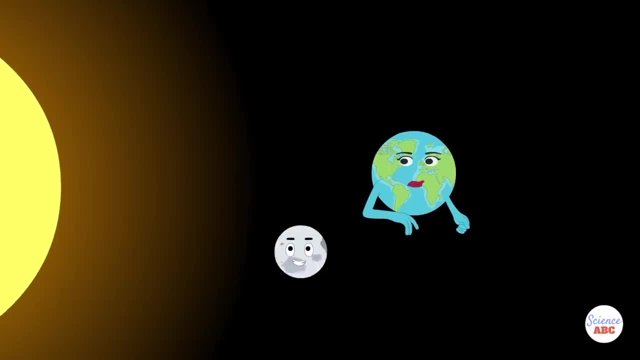 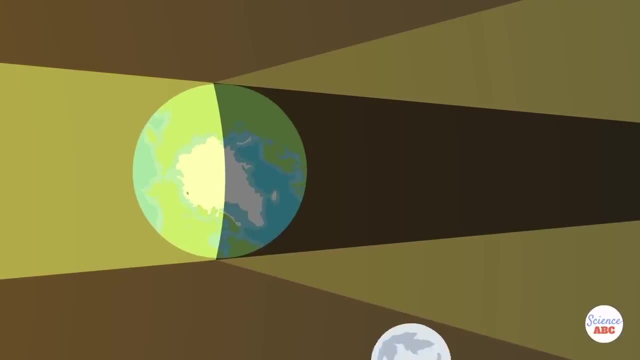 However, since the Earth rotates on its axis and also moves in its own orbit around the Sun, from our perspective, the Moon appears to orbit us every 29 days. Earth casts two types of shadows on the Moon: umbra and penumbra, when it is oriented between 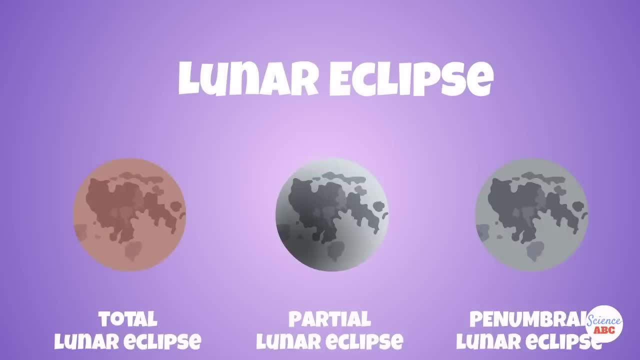 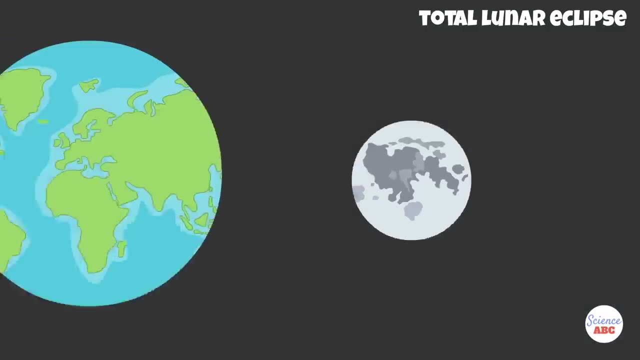 the Sun and the Moon. This is called a partial solar eclipse. Solar eclipses can be divided into three types, the first being a total lunar eclipse, The most picturesque and dramatic of all. a total lunar eclipse happens when the Moon, Earth and Sun are perfectly aligned, so that the Moon falls under the umbral shadow of our 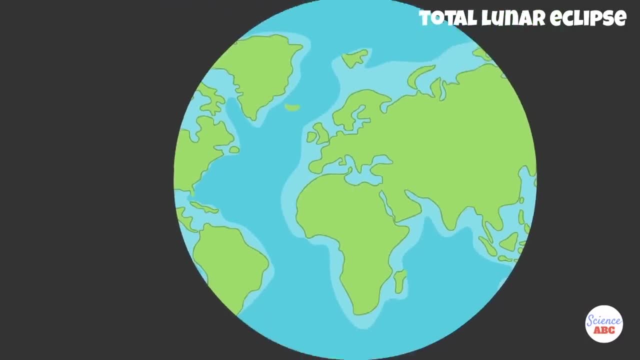 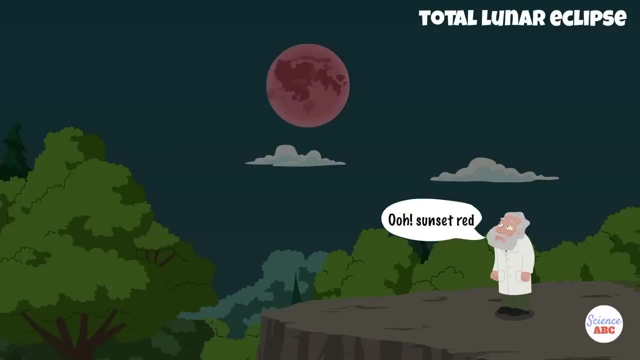 planet. During a total eclipse, Earth completely blocks any sunlight from reaching the Moon. Due to this, the Moon loses its characteristic whitish-gray color and becomes a sunset red. This happens due to refraction from the Earth's atmosphere. The shorter blue wavelengths of sunlight are scattered outward by the atmosphere. 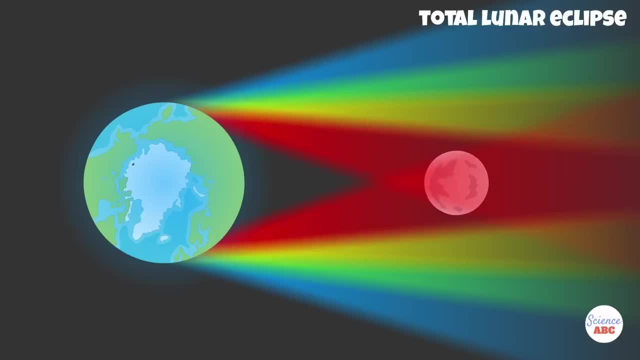 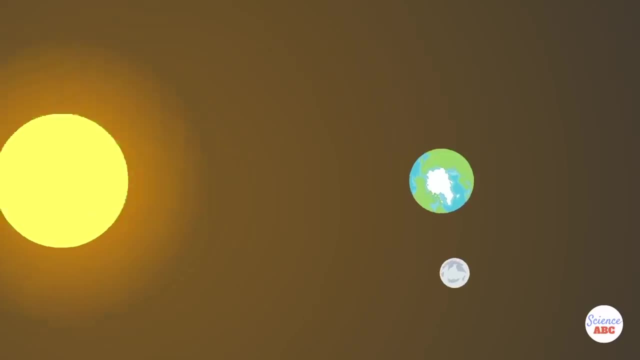 The longer red wavelengths are refracted inward towards the Moon, giving it a reddish tinge during a total lunar eclipse. Next is a partial lunar eclipse, which happens when the Moon, Earth and Sun align in such a way that only part of the Moon passes through the umbral shadow cast by the Earth. 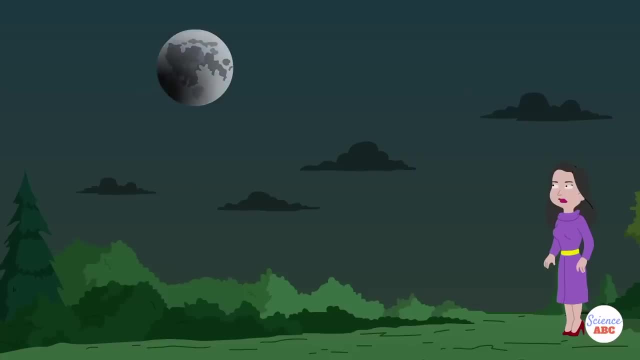 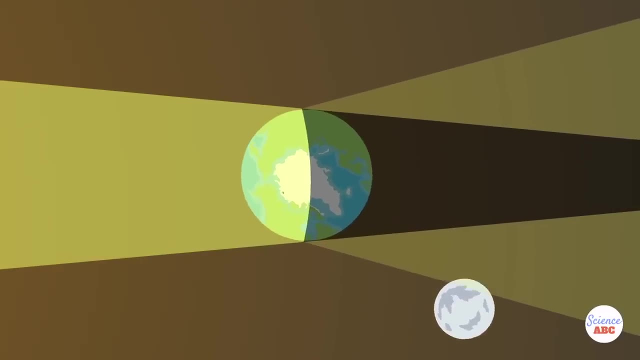 During a partial eclipse, you can see Earth's shadow covering a small part of the Moon's surface. Then there's a penumbra lunar eclipse, As the name suggests. you can see this type of eclipse when the Moon passes through Earth's penumbra shadow. 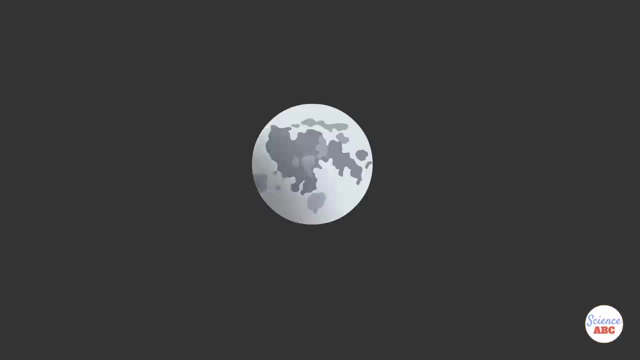 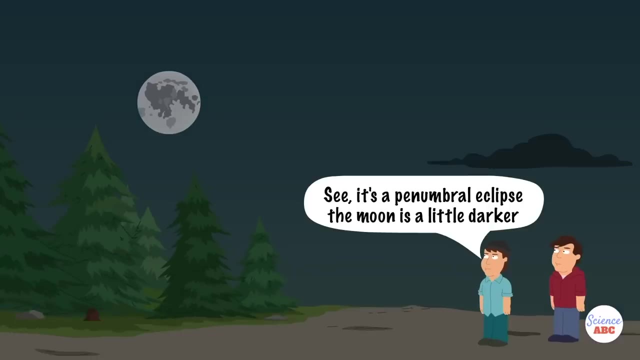 This celestial event is so subtle that many of us don't even notice it visually, as the Moon appears only slightly darker than its usual hue. So unless you are actively looking to observe the penumbra eclipse, it can be very easy to miss. 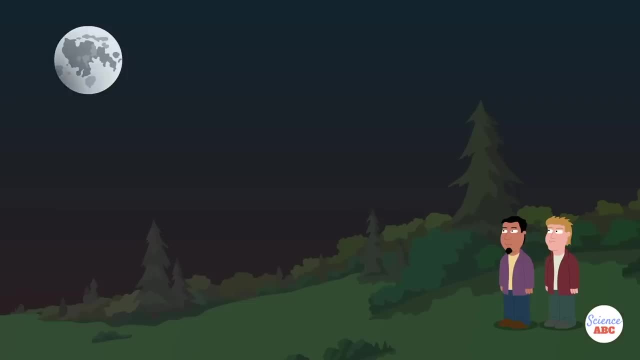 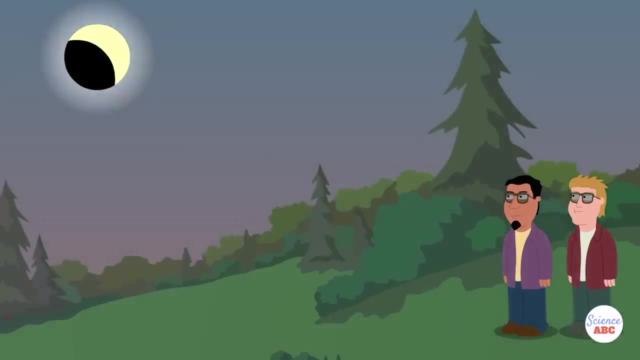 You can watch a lunar eclipse if you're on the nighttime side of Earth. and for those who are wondering, it's safe to watch a lunar eclipse with the naked eye. In contrast, it's highly dangerous to watch a solar eclipse with the naked eye. 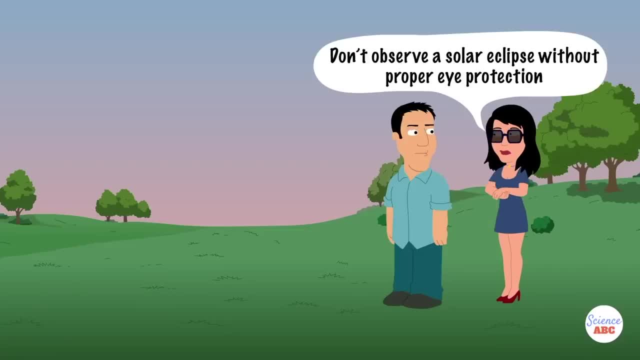 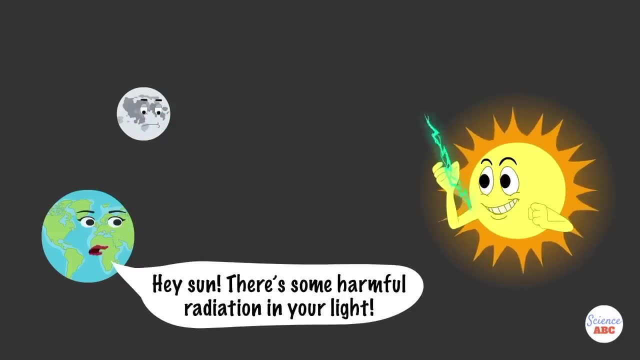 Observing a solar eclipse without appropriate precautions can potentially cause permanent eye injury. The light from the Sun that reaches the Earth consists of a broad range of radiation, from ultraviolet radiation at wavelengths longer than 290 nanometers all the way to radio waves existing in the meter range.